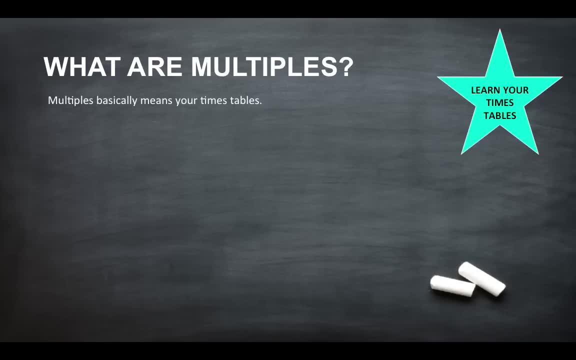 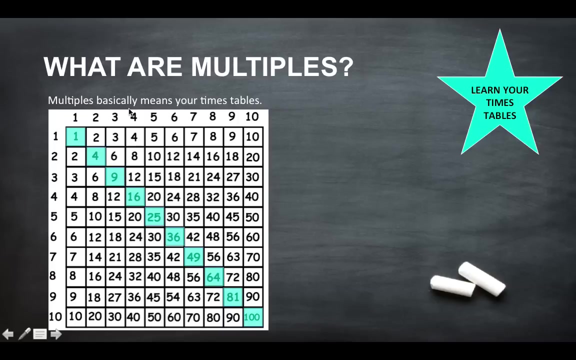 that you learn your times tables. So multiples basically means your times tables. So that's why I'm telling you to make sure you know your times tables off by heart. So I've given you a quick grid for your multiples. Ok, so, of course, you probably know all of these by now, But if you don't, this is just. 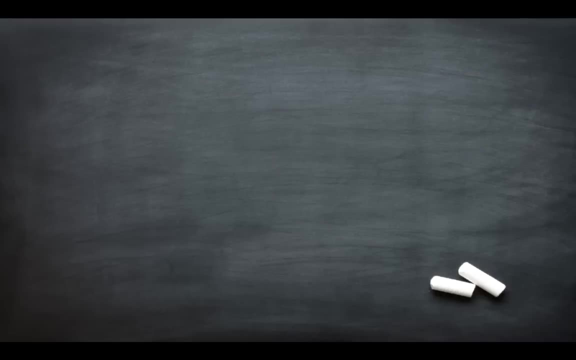 to recap and refresh your memory. Ok, so what are multiples? So the best way to teach you is by example. So the multiples of three. So think your three times tables, So you've got: one times three is three. two times three is six. three times three is nine, four times. 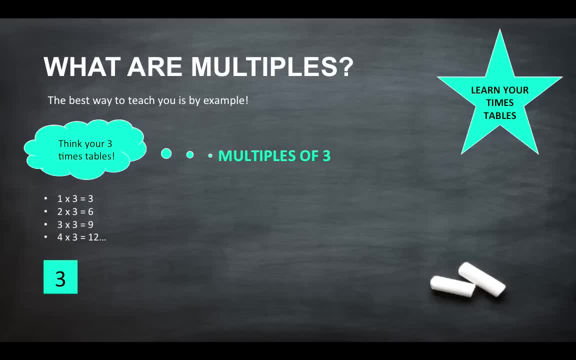 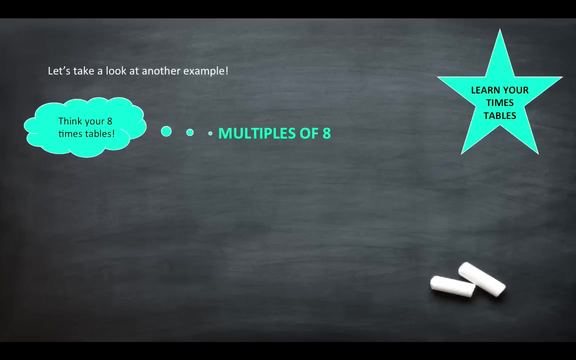 three is twelve and so on. So the multiples of three are three, six, nine, twelve, fifteen, eighteen, twenty-one and so forth. Ok, so it's basically just recalling and reciting your three times tables. Let's take a look at another example. So the multiples of eight. So again, think your eight. 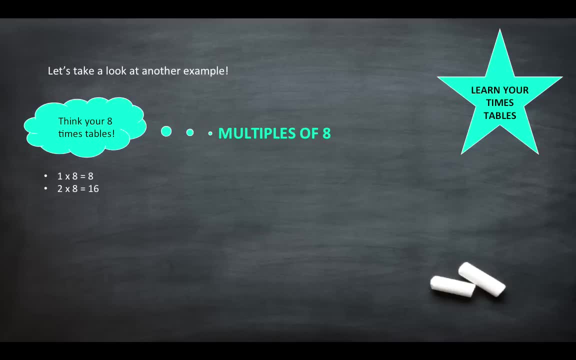 times tables. So we've got: one times eight is eight. two times eight is sixteen. three times eight is twenty-four. four times eight is thirty-two. So multiples of eight are eight, sixteen, twenty-four, thirty-two, forty, forty-eight, fifty-six and so forth. 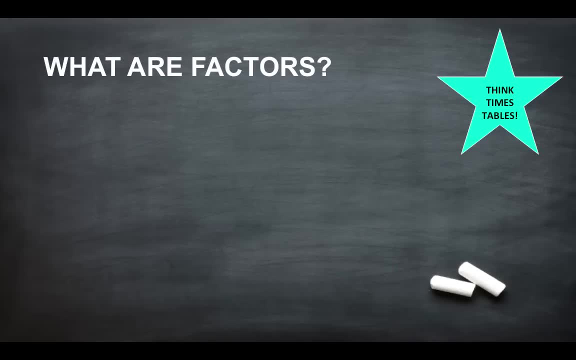 Ok, so what are factors? Ok, so again, you will also need to think your times tables. So factors are numbers that divide exactly into another number. So let me make this clearer: We're dealing with an example, So the factors of twelve. So you need to find all the numbers. 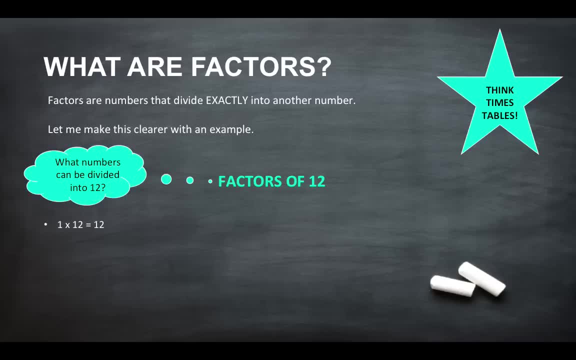 that can be divided into twelve. So we've got: one times twelve is twelve. two times six is twelve. three times four is twelve. So, in ascending order, the factors of twelve are one, two, three, four, six and twelve. Ok, because all of these numbers can be divided. 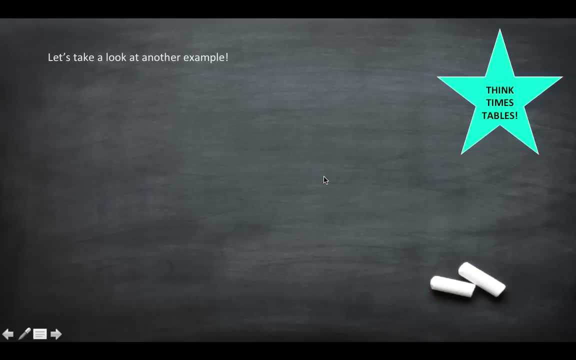 into twelve. So let's take a look at another example. So the factors of sixty. So what numbers can be divided into sixty? So we've got: one times sixty is sixty. two times thirty is sixty. three times twenty is sixty. four times fifteen is sixty. five times twelve is sixty and six. 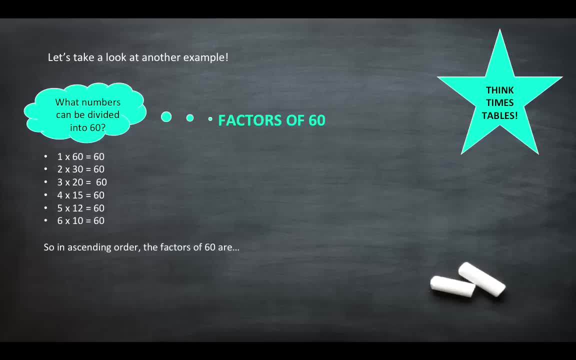 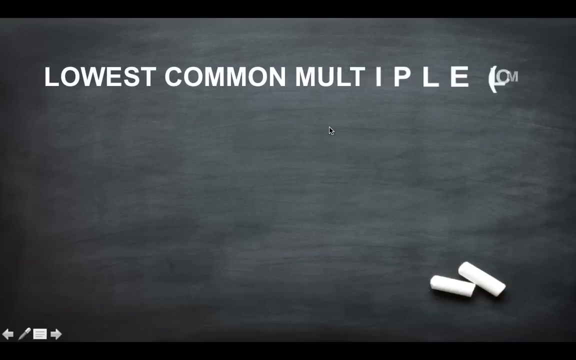 times ten is sixty. So, in ascending order, the factors of sixty are one, two, three, four, five, six, ten, twelve, fifteen, twenty, thirty and sixty. Ok, because all of these numbers can be divided into sixty. Ok, so the lowest common multiple, So the lowest. 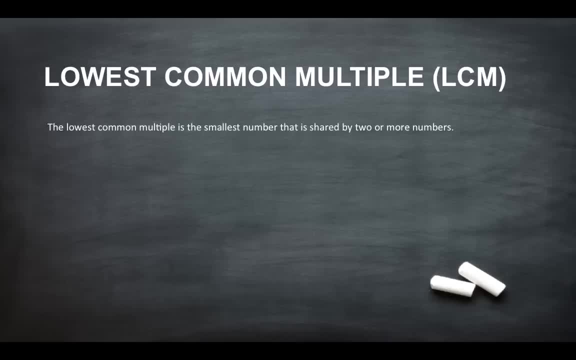 common multiple is the smallest number that is shared by two or more numbers. So let's use an example. So the lowest common multiple of nine and four. So first of all you need to do the first few nine times tables. So I've gone up to 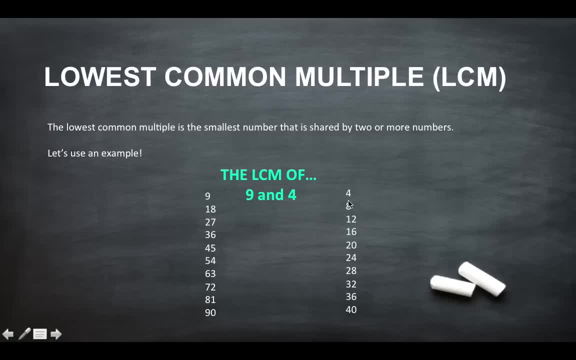 ninety. here And again you do it for the other number. So I've gone up to forty for the four times table, And then you need to find a number that they both share, which is the smallest common multiple. As you can see, both numbers have thirty-six And this is the lowest common. 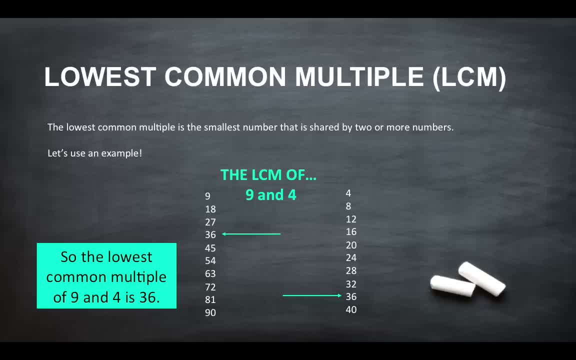 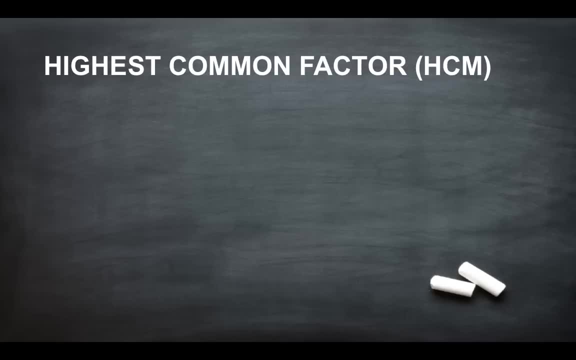 multiple that both nine and four share. So the lowest common multiple of nine is thirty-six, So the highest common factor. So to work out the highest common factor you need to work out the factors for each number and then work out which number appears for both, ie the 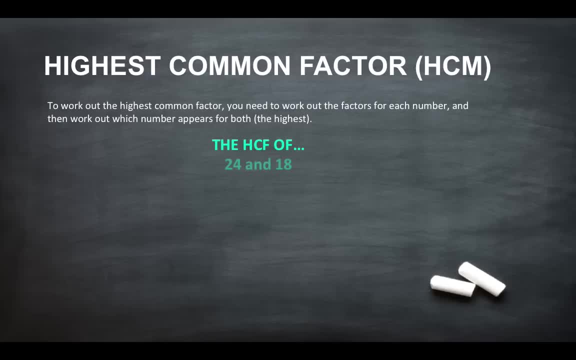 highest common factor, So the highest common factor of twenty-four and eighteen. So here are your factors. for twenty-four, So we've got one, two, three, four, six, eight, twelve, twenty-four. And for eighteen, we've got one, two, three, six, nine and eighteen. So you need to find. 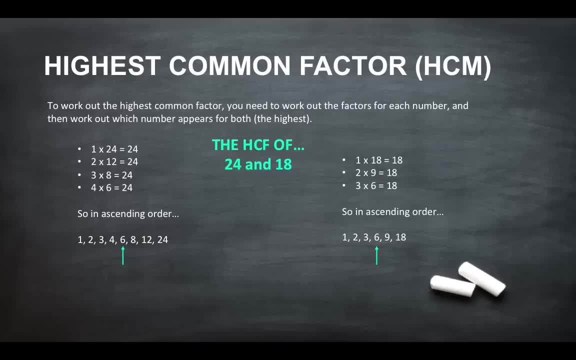 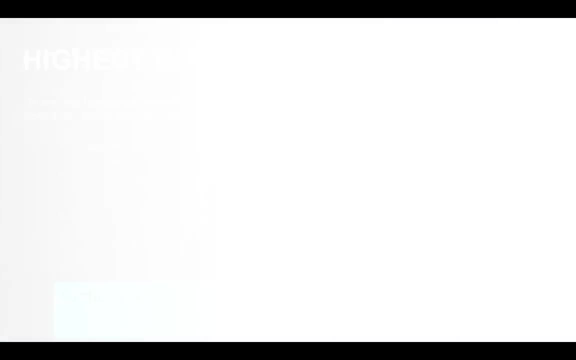 the highest common factor. As you can see, six occurs in both sets of numbers and it's the highest common factor that both of these numbers share. So the highest common factor of twenty-four and eighteen is six. Ok, so hopefully now you have a better understanding of multiples and factors For more practice. 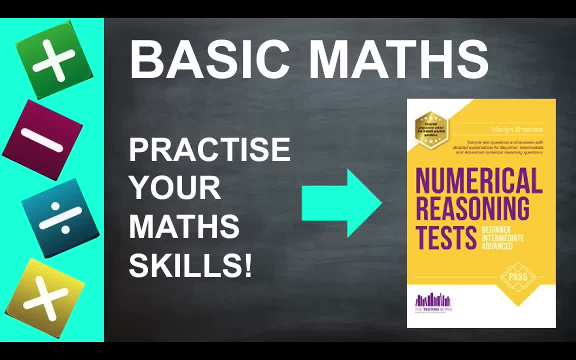 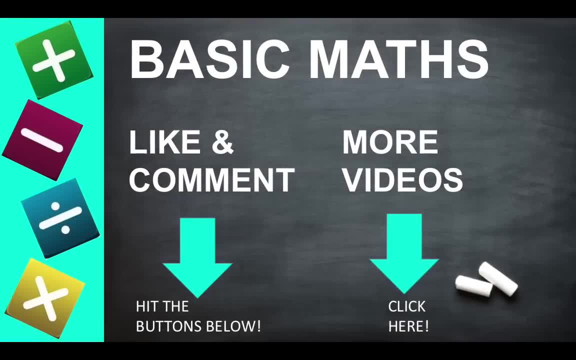 questions. you can go to the link in the description below For more questions. we have a fantastic guide on offer and can be purchased by clicking on the book cover, as shown now. Don't forget to like and comment on the video. If you have any other math videos you would like me to do, leave me your suggestion and I'll add it. 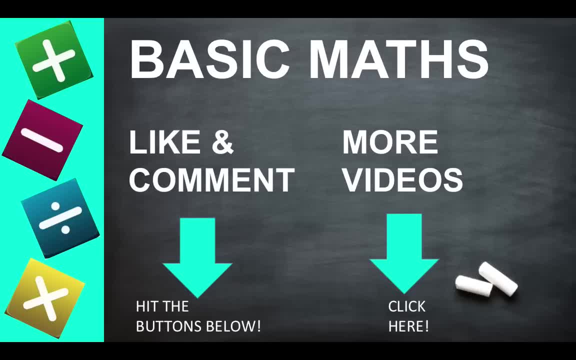 to my to-do list. For more videos, click on the click here button and hover over the coloured rectangle boxes to be directed to one of my other short mathematical videos. That's it from me. Stay updated with a whole range of my basic math videos. I'll see you in the 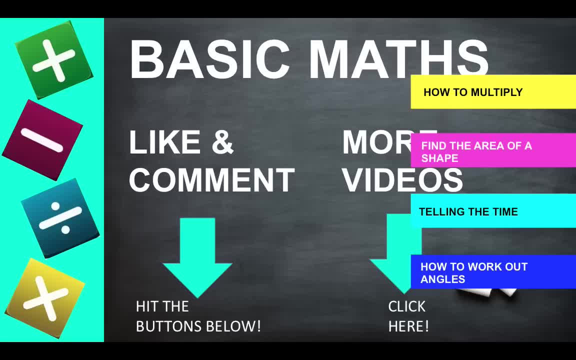 next one. I wish you the very best of luck and thank you for watching. 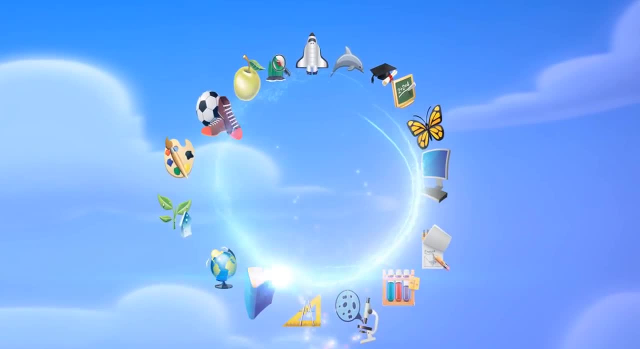 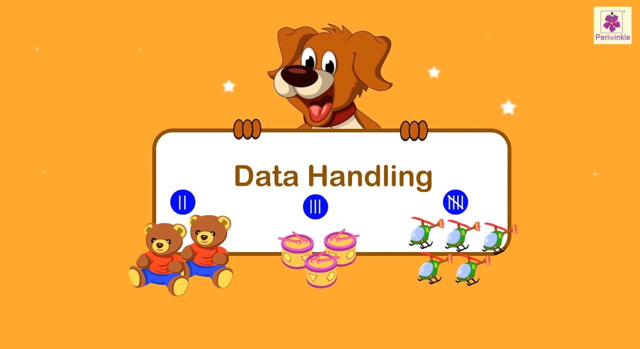 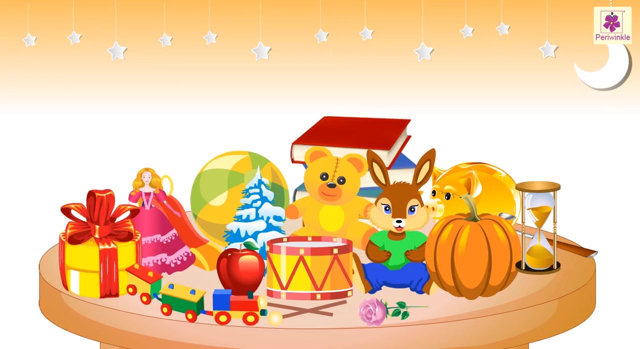 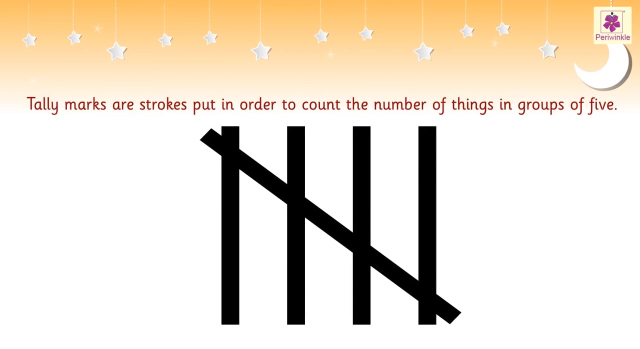 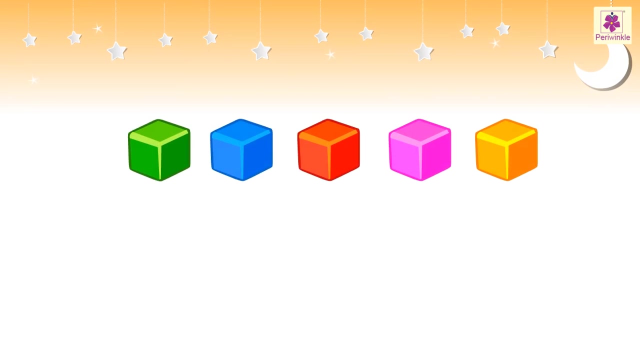 Data Handling. Counting of many objects can be difficult. In order to easily count many objects and keep a score, we use tally marks. Tally marks are strokes put in order to count the number of things in groups of five. We draw one straight line for the first four objects. 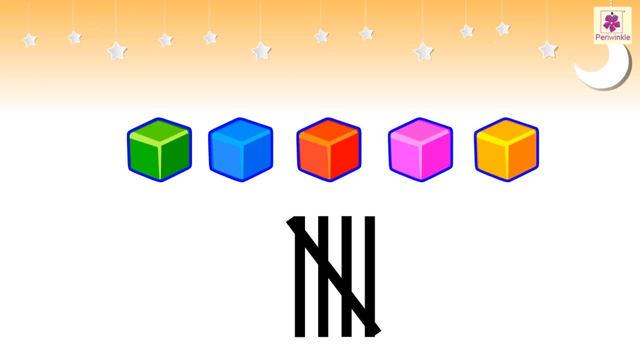 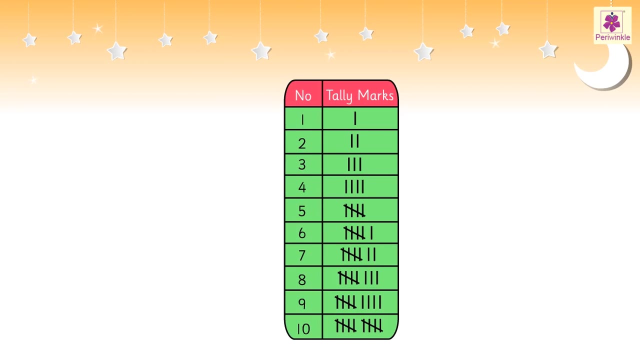 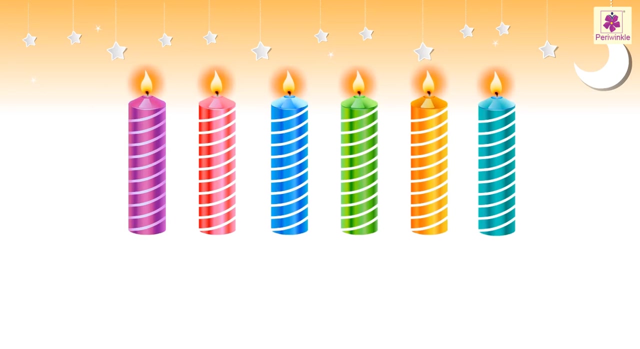 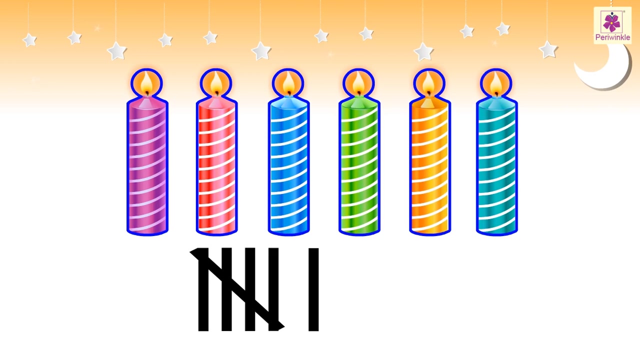 The fifth object is represented by a slant line across the previous four lines For numbers from 1 to 10, the tally marks are represented as given here. Let us count the number of candles using tally marks 1,, 2,, 3 and 4 straight lines and a slant line across, and then again a one. 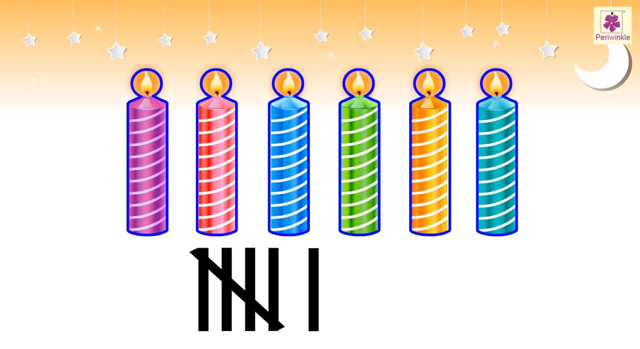 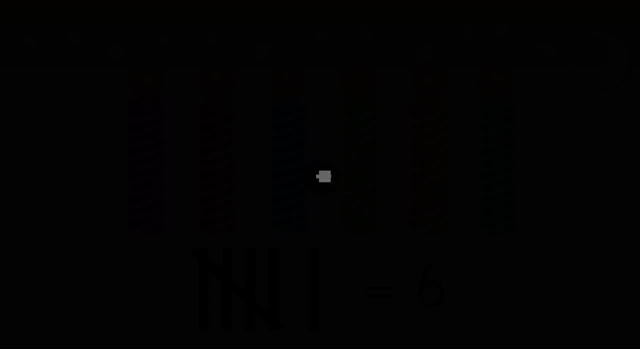 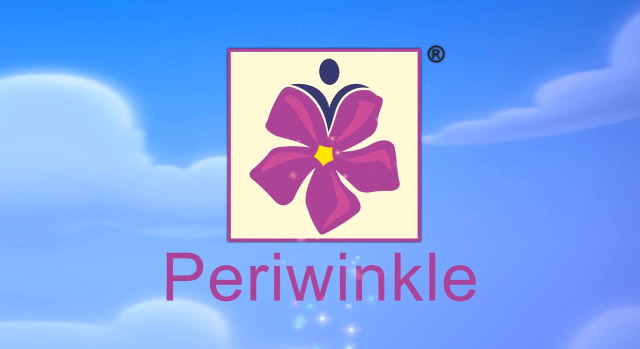 Hence we get the number of candles as 6.. The answer is correct. Let us know if we have any questions. Let us know the correct answer in the comments. Thanks, Let us know if you have any questions. Let us know if we have any questions.